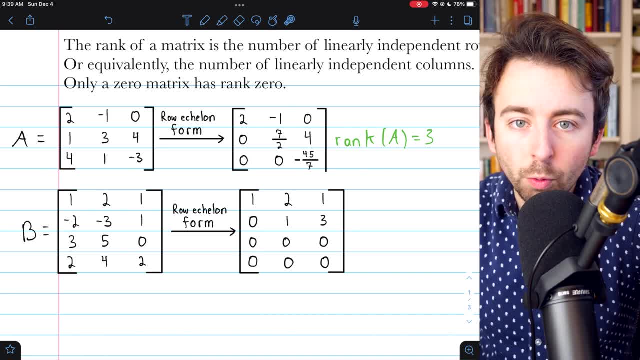 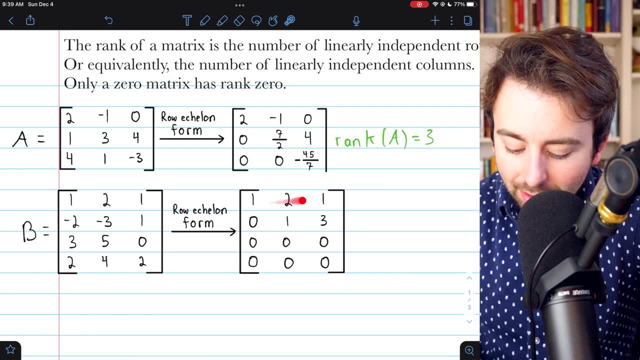 this is what we get. The number of linearly independent rows in B is the number of non-zero rows in the row echelon form. In this case there are two non-zero rows, so the rank of B is 2.. Some matrices are simple enough. 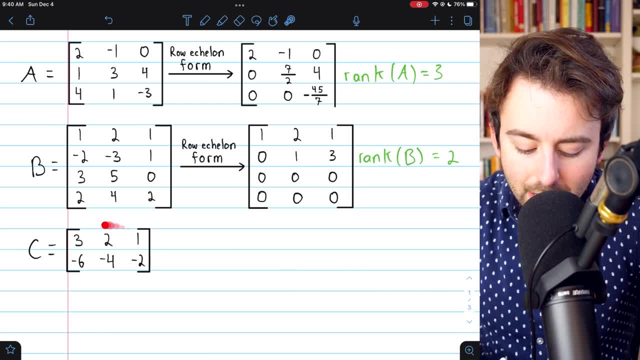 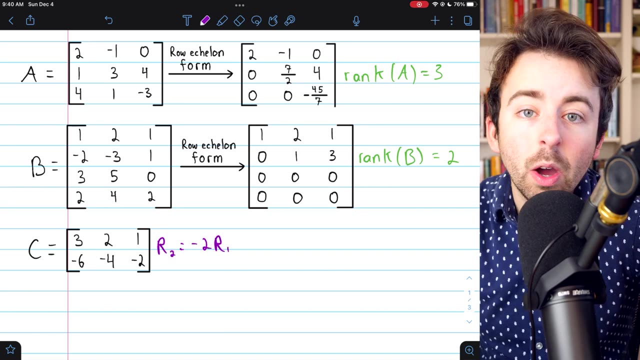 that we don't need to put them in row echelon form. This matrix C is not the zero matrix, so it does have a positive rank. but I notice the two rows are not independent. The second row is simply equal to negative 2 times the first row, so C has only one independent row and its rank. 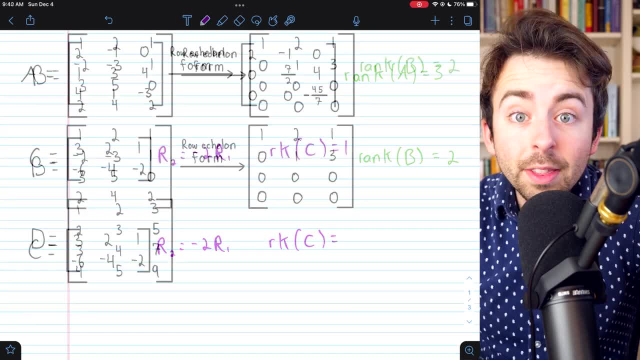 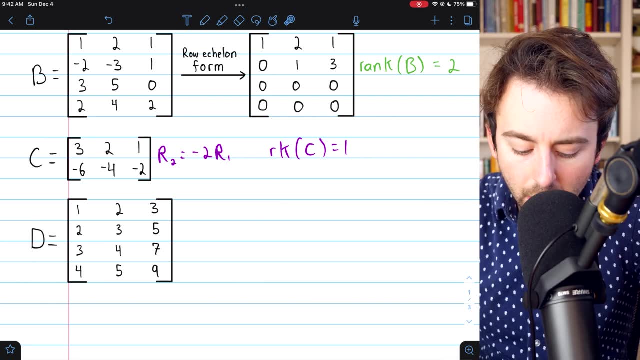 which we could also denote like this, is equal to 1.. This matrix D has fewer columns than it has rows, so it may be simpler to look at the columns. We notice the first two columns are linearly independent. There's no way to multiply column 1 to get column 2.. However, column 3 is a linear. 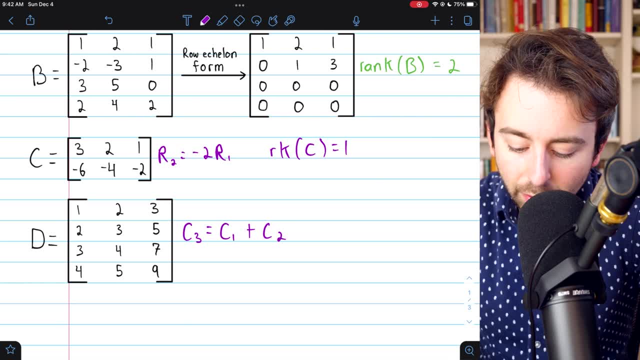 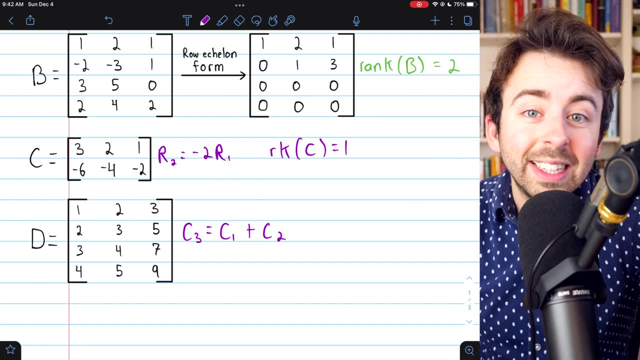 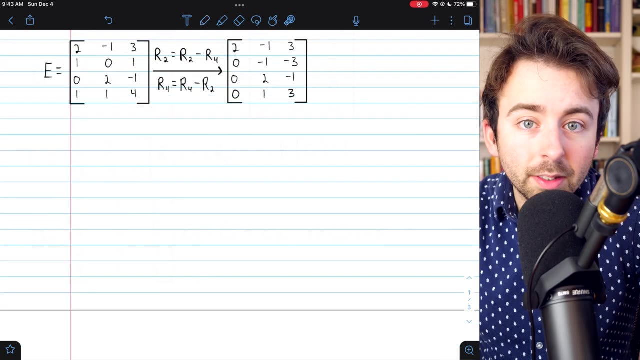 combination of the first two columns. In fact, if we just add column 1 and column 2, that gives us column 3. So the matrix D has only two linearly independent columns, and we would say that the rank of D is equal to 2.. If all else fails, we can always put the matrix into row echelon form. 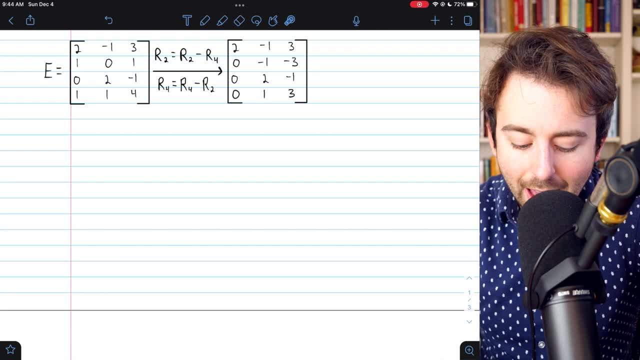 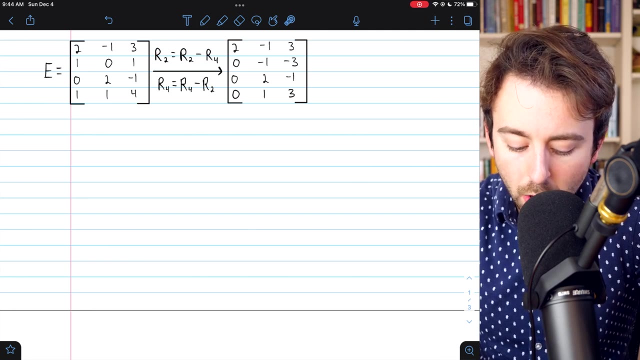 and count the non-zero rows. Let's do one more example of that with this matrix E. We want to make the entries below each leading entry equal to the number of rows in the row echelon form. To get that we'll set row 2 equal to row 2 minus row 4, so those 1s will cancel out To get rid of. 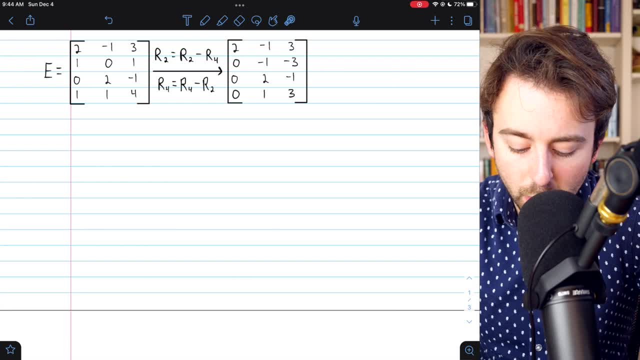 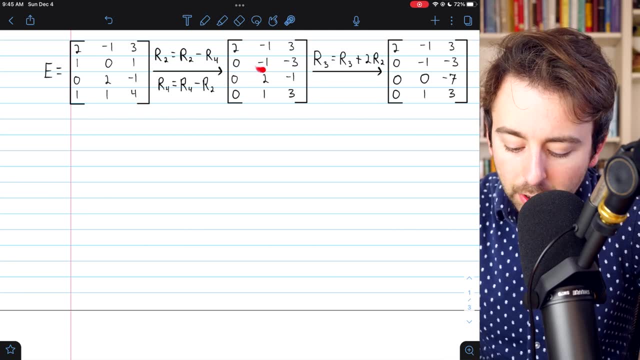 this one, we will subtract row 2 from row 4, to again cancel out the 1s. That gets us here. We have 0s below the 2, like we want. Now we want to get 0s below the next leading entry of negative 1.. 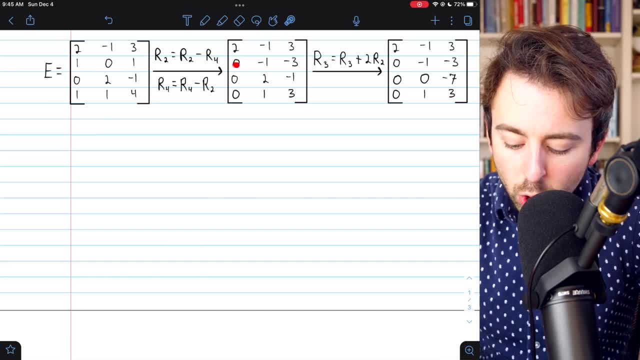 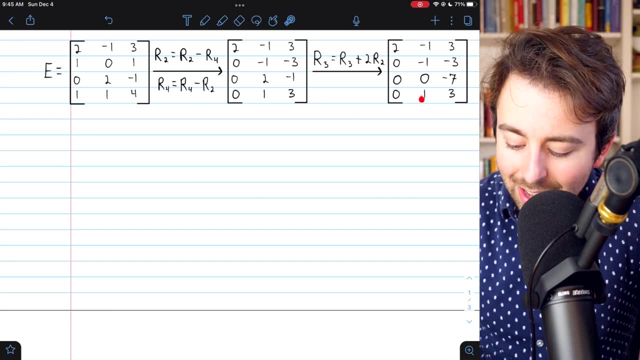 To make this 2 equal to 0,, we'll add two copies of row 2.. We'll add row 2 into this third row, and that gets us here. Now we also want to get rid of this one that's below the leading entry of negative 1,, and in order to do that, we'll simply add row 2. 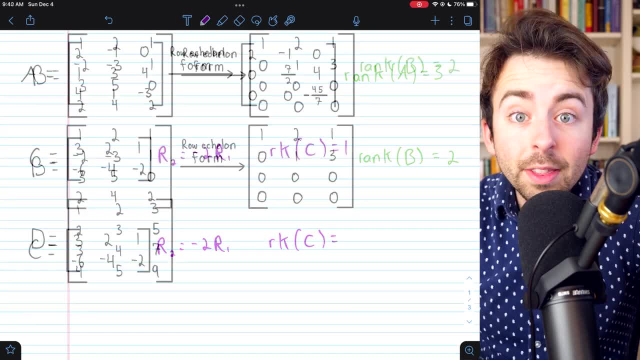 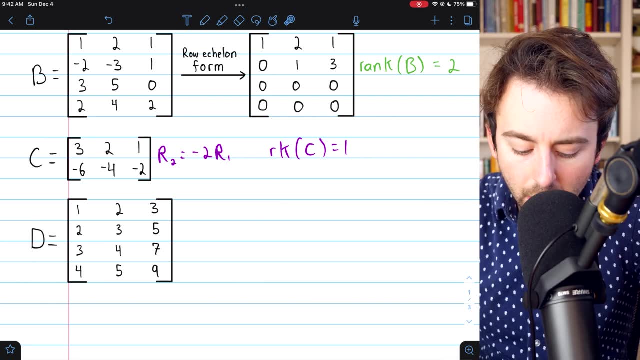 which we could also denote like this, is equal to 1.. This matrix D has fewer columns than it has rows, so it may be simpler to look at the columns. We notice the first two columns are linearly independent. There's no way to multiply column 1 to get column 2.. However, column 3 is a linear. 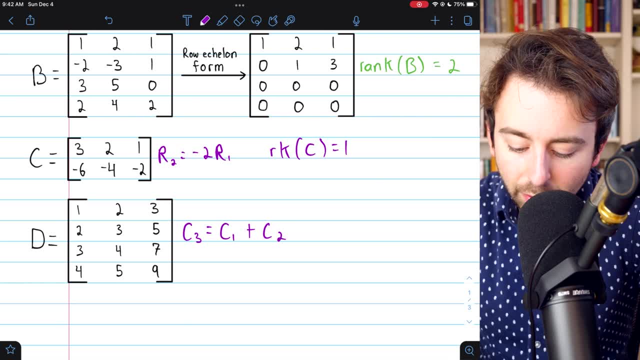 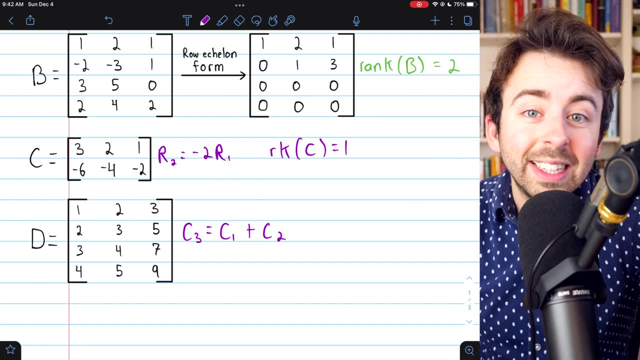 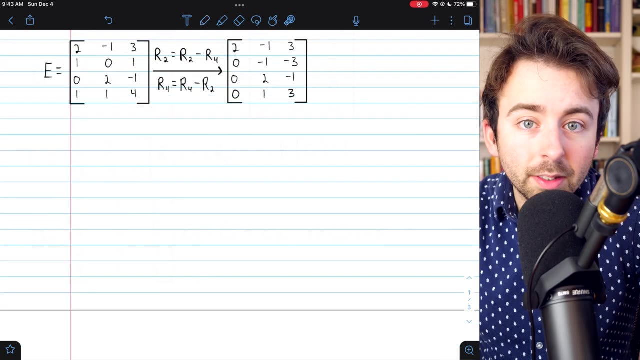 combination of the first two columns. In fact, if we just add column 1 and column 2, that gives us column 3. So the matrix D has only two linearly independent columns, and we would say that the rank of D is equal to 2.. If all else fails, we can always put the matrix into row echelon form. 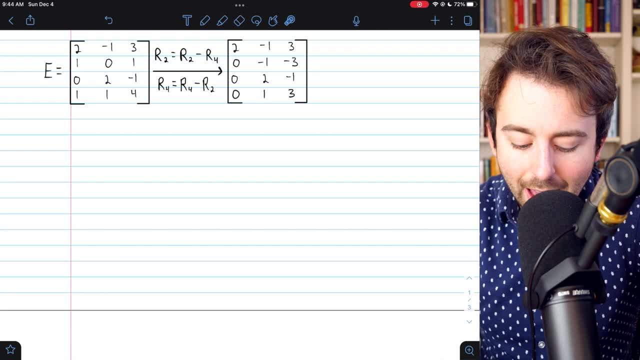 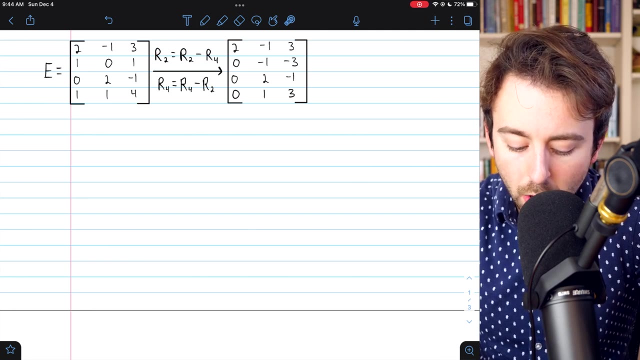 and count the non-zero rows. Let's do one more example of that with this matrix E. We want to make the entries below each leading entry equal to the number of rows in the row echelon form. To get that we'll set row 2 equal to row 2 minus row 4, so those 1s will cancel out To get rid of. 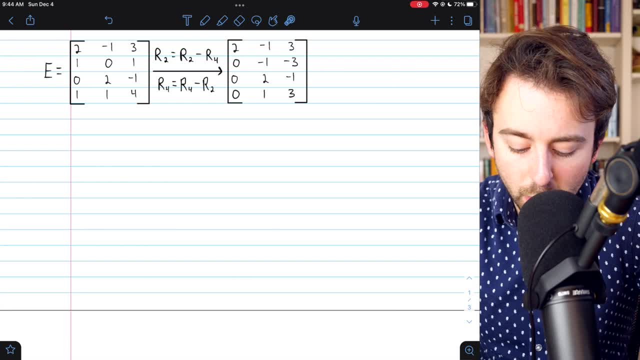 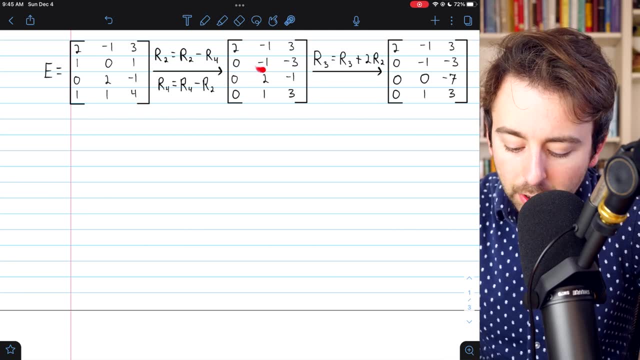 this one, we will subtract row 2 from row 4, to again cancel out the 1s. That gets us here. We have 0s below the 2, like we want. Now we want to get 0s below the next leading entry of negative 1.. 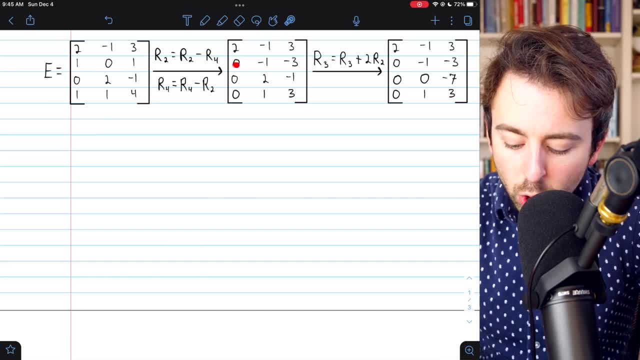 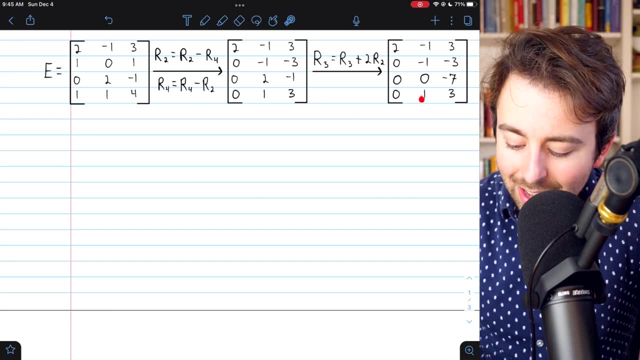 To make this 2 equal to 0,, we'll add two copies of row 2.. We'll add row 2 into this third row, and that gets us here. Now we also want to get rid of this one that's below the leading entry of negative 1.. And in order to do that, we'll simply add row 2. 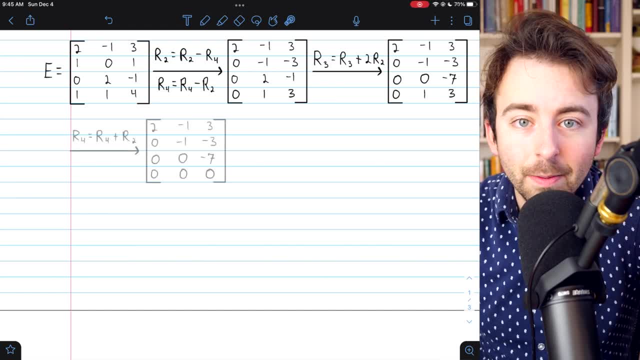 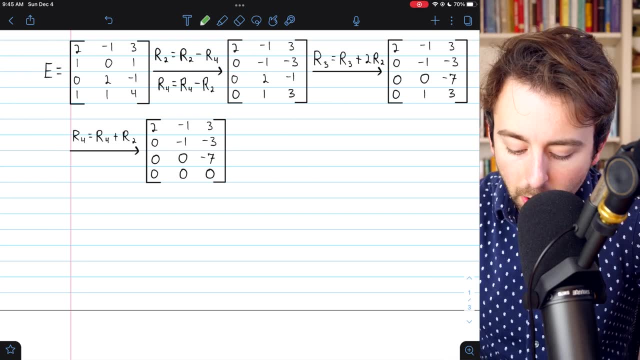 to row 4, which will eliminate row 4 completely. So row 4 is all 0s and we can see we are now in row echelon form and there are three non-zero rows. Thus the rank of E equals 3..